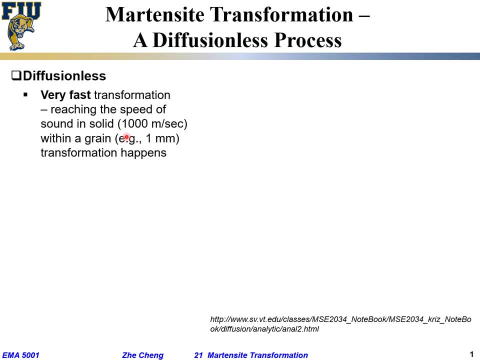 find is it's actually reach the speed of sound wave propagate within the steel, the solid it can propagate as fast as 1000 meter per second. if you think, if i have a typical palm sized material, that the whole material would transform within, wow, one millisecond. really, really, really fast okay. 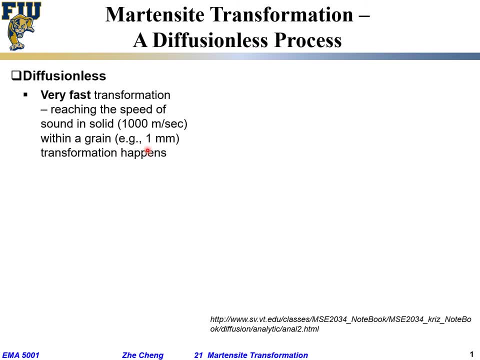 within the grain. well, fast, what we are showing here are the change of diffusion coefficient versus temperature. we said people find that quite often they would happen occur within one microsecond, well, within one millisecond. sometimes within one microsecond if we think the the time scale that would not allow a change in composition. 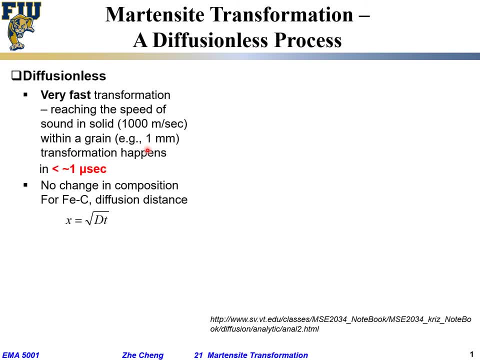 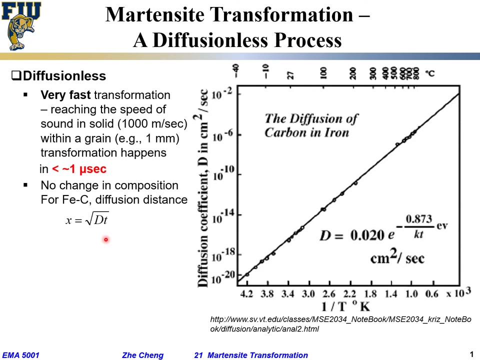 it will not allow a changing composition because the diffusion length, the square root of dt, d for diffusion coefficient, t for time, the square root of dt, is our typical diffusion length. it's very, very short. if we look at the phase, the not phase diagram, the diffusion coefficient versus temperature curve, and let's look at a number of 10 to the power of. 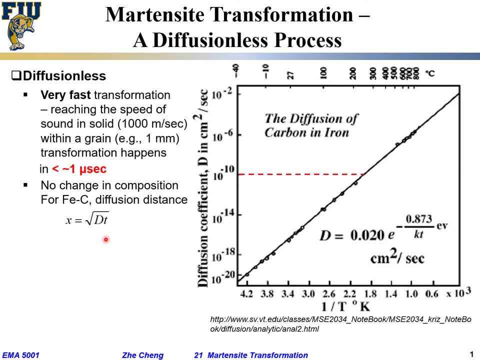 a negative 10 right, which is a very small number. the corresponding temperature would be between 200 to 300 degrees c. that's kind of like when you quench from 700 red hot to something like 200. okay, you don't have to go to the room temperature just when you quench the. 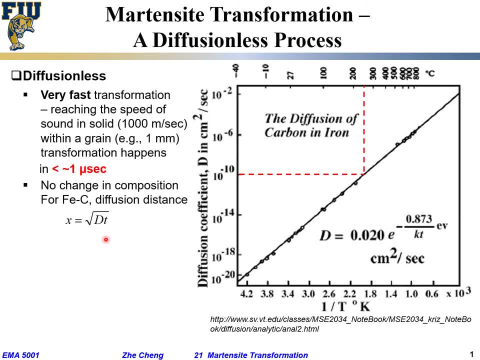 inside may take some time. let's say quench to 200, the diffusion coefficient is roughly 10 to the power of negative, 10 in the unit of centimeter square per second. then if we say the whole process happens within one microsecond, what's the diffusion length? if you do an estimate, 10 to the power of negative, 10 times microsecond is 10. 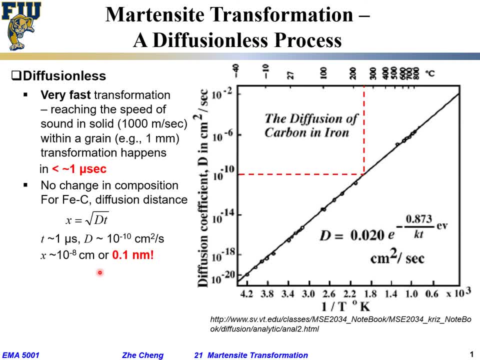 to the power of negative. what 6 right so combined, is 10 to the power of negative 16.. and you take the square root, you get the 10 to the power of negative 8 centimeters. 10 to the power of negative 8. 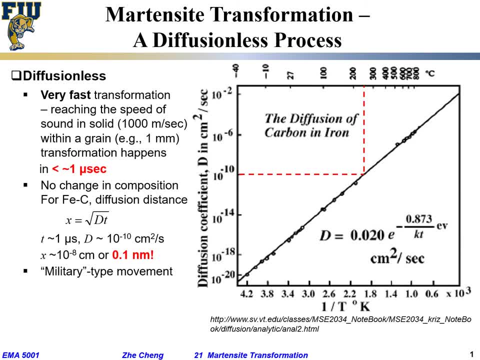 centimeters. that's how much. that's even 0.1 nanometer, which means within this short period of time the carbon comes at mostせntimeter. there is a lot of potential in addition to this short period of time the carbon can at most. this short period of time, the carbon can at most. 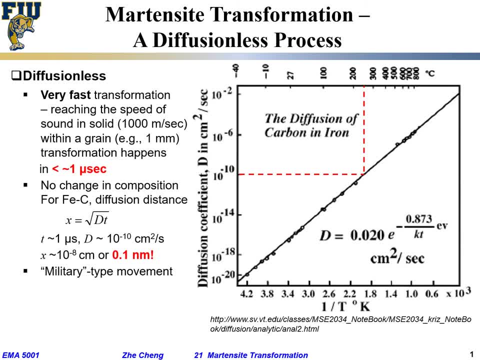 diffuse how much? 0.1 nanometer, that's much less than that. you are within a lattice parameter, which means the carbon cannot even move beyond the one unit cell, which means what the carbon go or does not go does not go, it's carbon is still in there. whatever carbon there, it doesn't move. 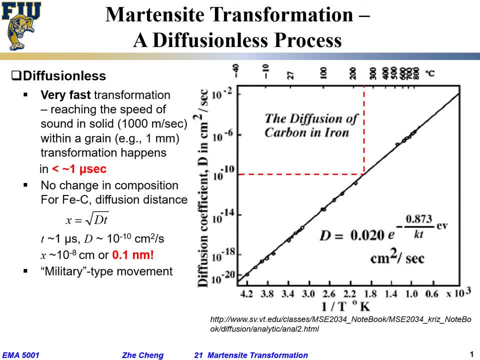 and the transformation process is already finished very, very fast. and people say it's so-called military type. okay, military type movement, which means, okay, the atoms move fast, and the atoms moves in a coordinated fashion. not in the coordinated fashion- i don't say they move in the same speed, it depends- but they are in a high speed. 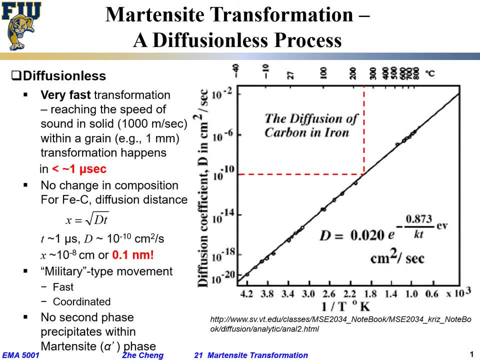 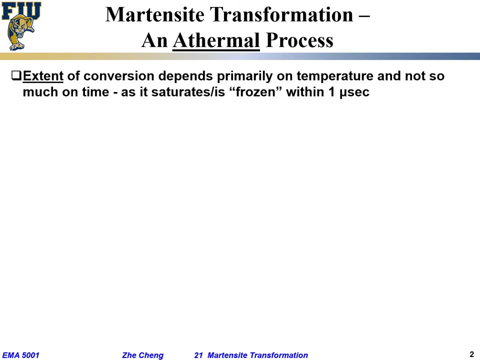 in a highly coordinated fashion, not random, otherwise you cannot achieve it. okay, and what people observe is quite often: there's no secondary precipitate within the martensite transformation, within the martensite form. there's no cementite within the martensite phase. okay, so in terms of 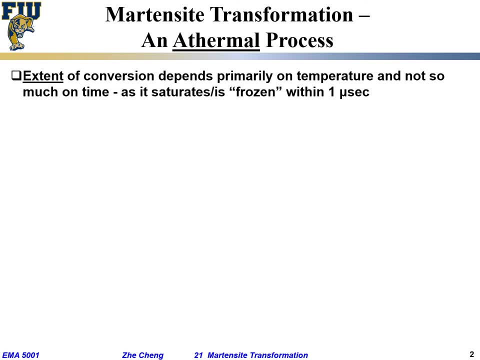 the feature of how does it change with time and temperature? people quite often call this process A3 thermal. a thermal means it's not exactly similarly activated. it doesn't get faster by higher temperature. okay, and actually people observe this. the extent of transformation depends on temperature, not so much on time. if we're going to plot on the left, 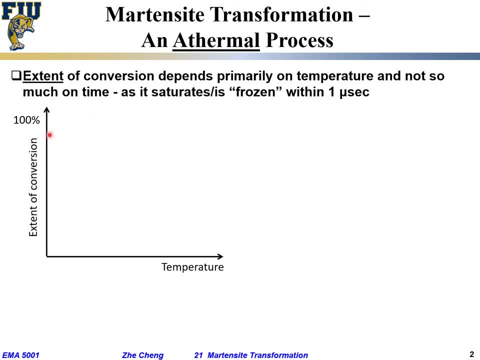 side, the change in extent of conversion versus temperature. what people observed is: at higher temperature towards the right, the extent of transformation would be zero. but as the temperature goes lower and lower, depending on how low we quench, the transformation increase, quickly increase and the saturation and the beginning of that.